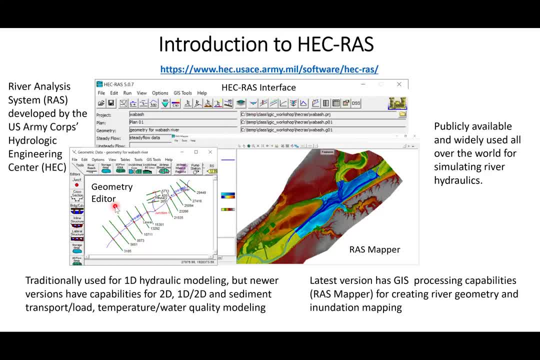 creating HEC-RAS goes into creating this geometry file, and this geometry file is created using RasMapper. Traditionally, HEC-RAS has been used to perform 1D hydraulic modeling, but the newer versions of HEC-RAS will allow you to perform two-dimensional modeling. 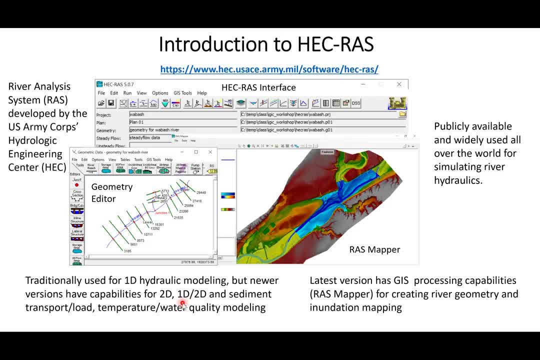 It will also allow you to perform a combination of one-dimension and two-dimensional modeling and you can also do sediment transport or load. And you can also do sediment transport or load. For this module. we will be doing only temperature or water quality modeling. 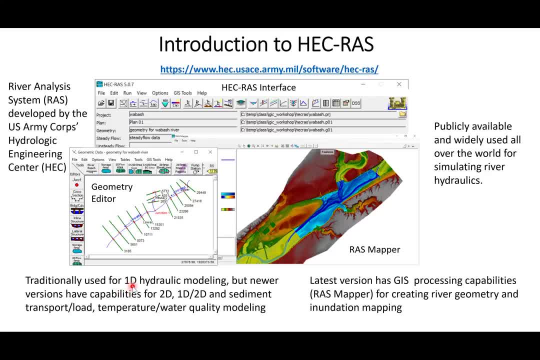 but in this module we will be doing only one-dimensional hydraulic modeling. As I said earlier, we have to create this geometry file and in the older versions of HEC-RAS there was no GIS interface. We had to use an external GIS software, such as HEC-GORAS, to create this geometry file. 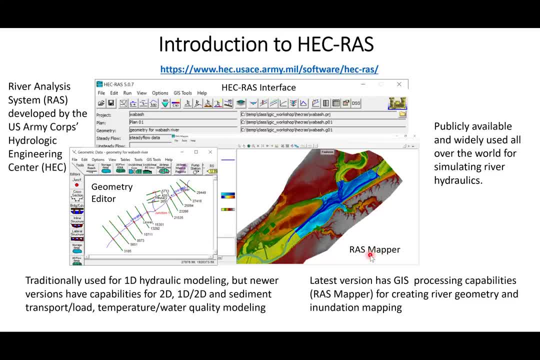 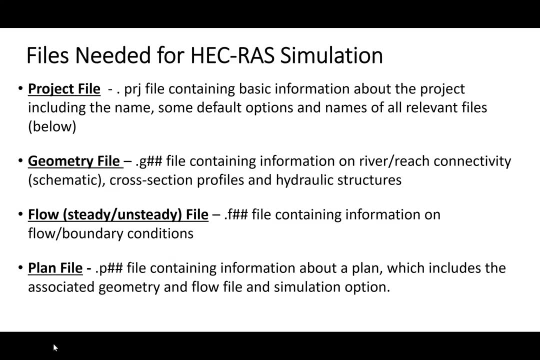 But the newer version of HEC-RAS has this RasMapper. but the newer version of HEC-RAS has this RasMapper which we can use to create a geometry file. so we don't need any other external GIS software. we can do everything in HEC-RAS. when we create a HEC-RAS model, basically we create these four. 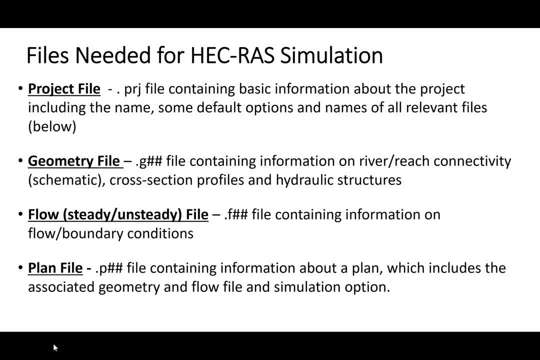 files, and these are the minimum files that you need to run a hydraulic simulation. the first file is this project file. it has an extension of prj. for example, if we name our project as wabash, the project file will have a name wabashprj. it contains information about the project. 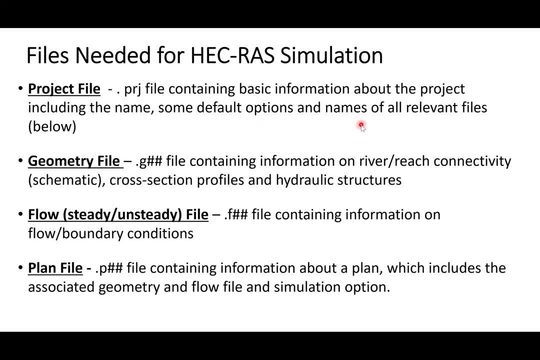 including its name, some default options and the name of all the relevant files. and these files are what the geometry file is: flow file is and plan file. a geometry file will have the same name as the project. so if we named our project as wabash, a geometry file will have wabashg and these means the numbers. so the first: 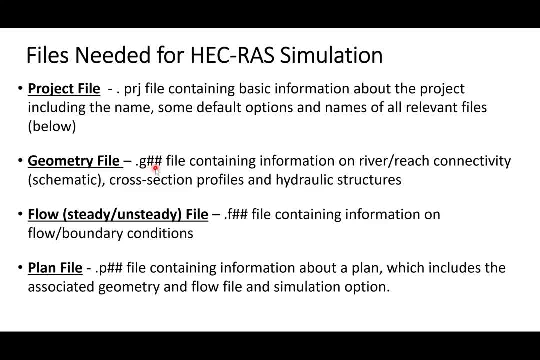 version of geometry file will have g01.. so the first version of geometry file will be named wabashg01 and it will primarily contain information on river or reach connection, Burma and Java, or you can think of that as a schematic of our river system. it will also contain 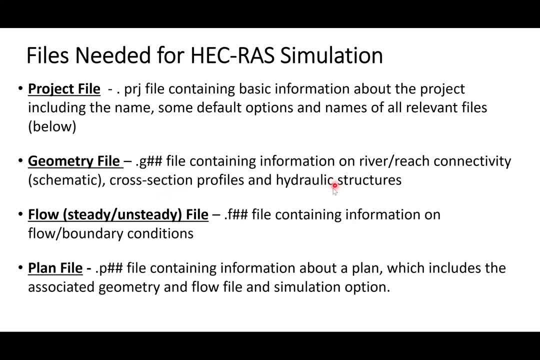 information on cross-sectional profiles and any hydraulic structures that are included in the model. the next file will be the flow file and, depending on what kind of simulations we are performing- whether it's a steady state or unsteady state- it will be either named steady flow file or unsteady flow file. it will 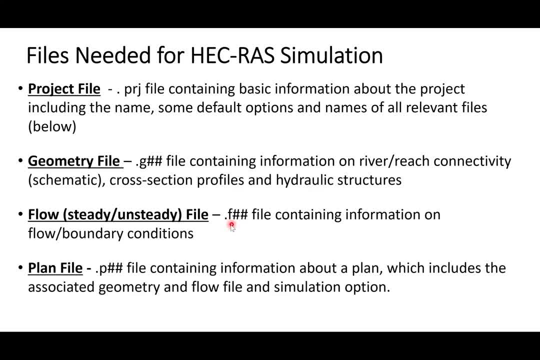 have the same name as our project and the extension will be f and number. so the first version of flow file will have WABASHF01 and this file will mainly contain information on flow and boundary conditions. and finally, when we create and run a simulation, a plan file gets created and that will have an 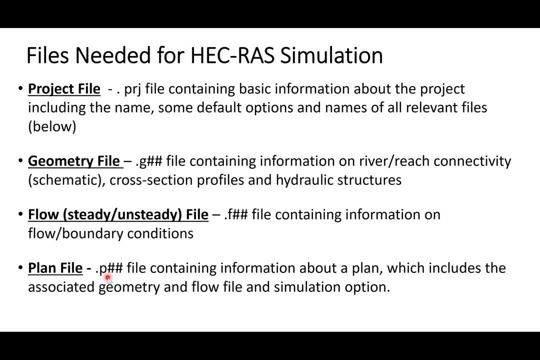 extension of P and a two-digit number. so the first file we will have is VBAS and then this box, the section will contain important name as f version of plan file will have wabashp01 and it will contain information about a plan which mainly includes the geometry and flow file associated with. 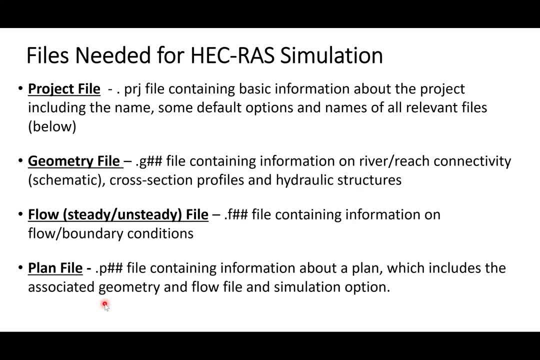 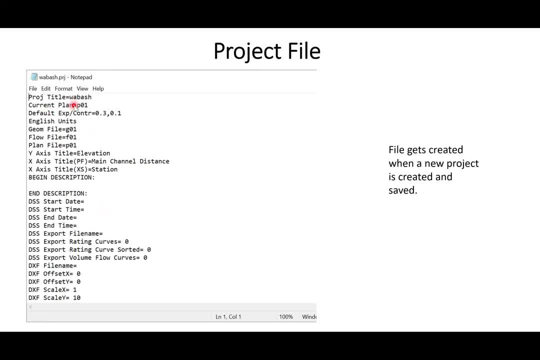 the simulation and the simulation options that we have selected. this is how the project file looks. it is a simple text file. as I mentioned, it will have the name of our project, what the current plan, geometry and flow files are and all the default options included in the model when we create a new. 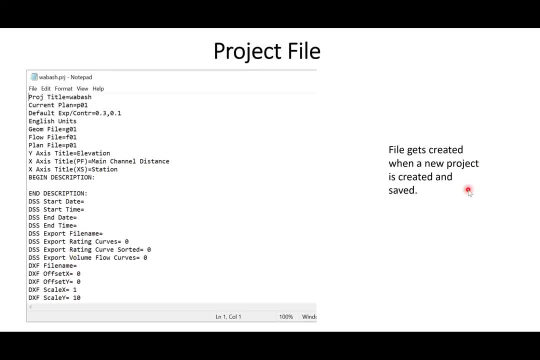 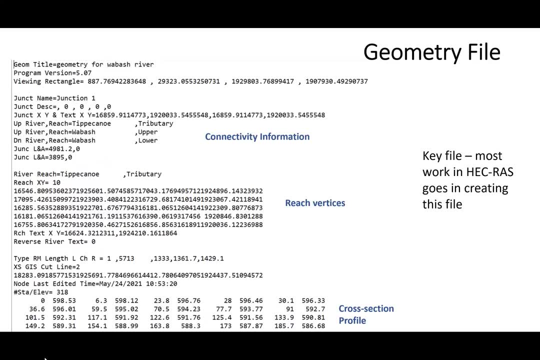 project and save it, a project file will automatically get created and it will be saved as project name: dot PRJ. after we create project file, the next important file that we create is the geometry file, and that is what you see here on this slide. this is again a text file and this file 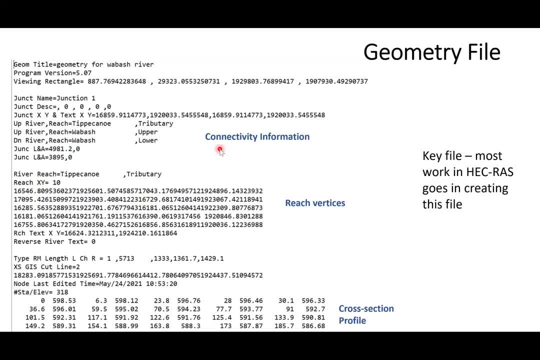 as I mentioned earlier, it will contain information on reach or reverse connectivity that you see here. it will contain information on how the reach looks like. so what you see here are all the points that are describing the Reaches, and then, finally, it will contain information on cross-sections and 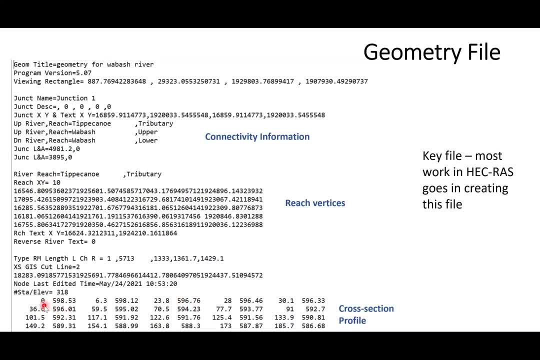 hydraulic structures. so what you see here is station and elevation pairs, and these pairs describe the top and bottom components, which is a great tool for check in three-dimensional structure of our cross section. and this is the most important file that we are going to create and it takes most of the time involved in. 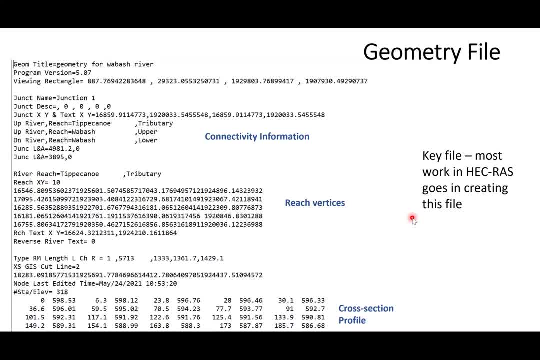 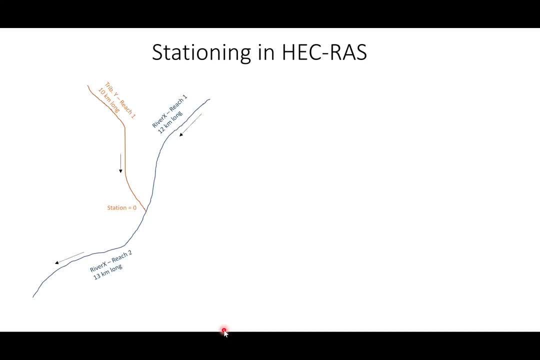 setting up a HEC-RAS model, and that is what we will look at in the next few slides. Before we get into how to create the geometry file, we need to understand how information is stored with river geometry in HEC-RAS- An important 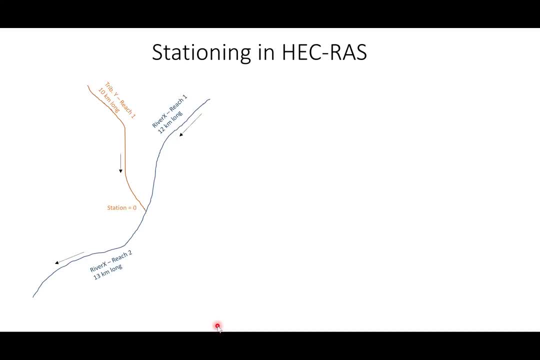 concept that HEC-RAS uses is stationing. so let's understand what that means. What you see here on the left is a river system. it has this main river and then there is a tributary joining to this main river. Since we have a tributary, 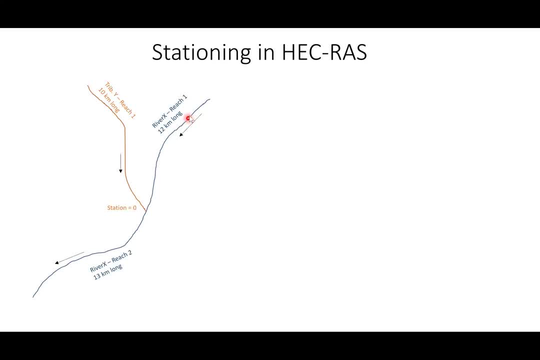 here the river gets divided into two reaches, so we are calling this river as river X. this is reach 1. it is 12 kilometers long. this is the downstream reach, reach 2 on the same river X, and this is 13 kilometer long. and then we have the 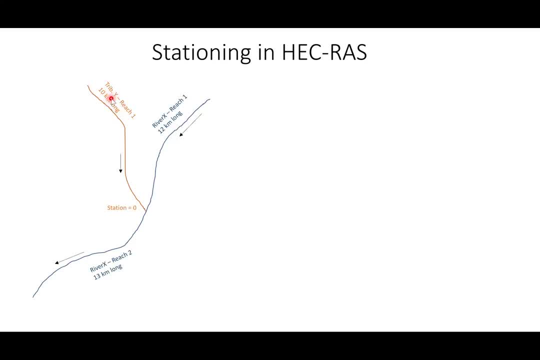 tributary, which we are calling it as tributary Y, and since this is the only reach, this is our reach 1, and this is 10 kilometer long. So now that we know the lengths of each of these reaches, the way stationing works in HEC-RAS. is that the 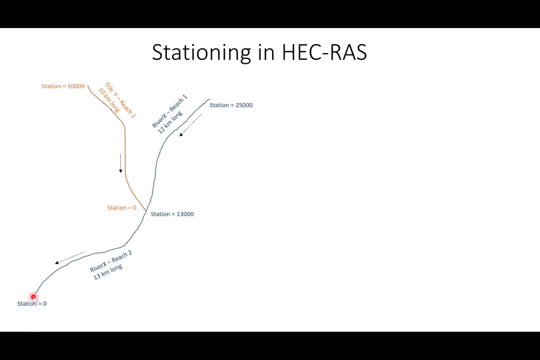 most downstream point will have a station of 13.6 miles long. So let's zero, and that stationing increases as we go upstream along the river. so in this case this reach is 13 kilometer long. so that's why, when you reach here at the 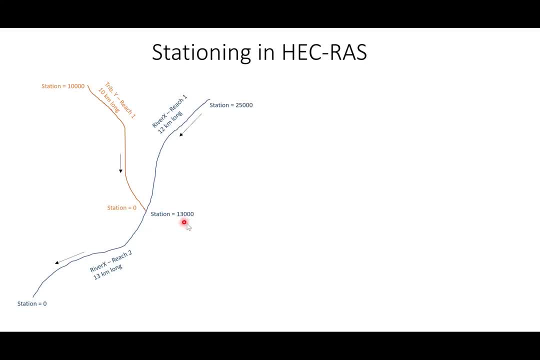 junction, the stationing for this river will have a value of 13,000, so in this case we can think of this as 13,000 meters. and as we go up, since this reach is 12 kilometer long at the most upstream location, the stationing is: 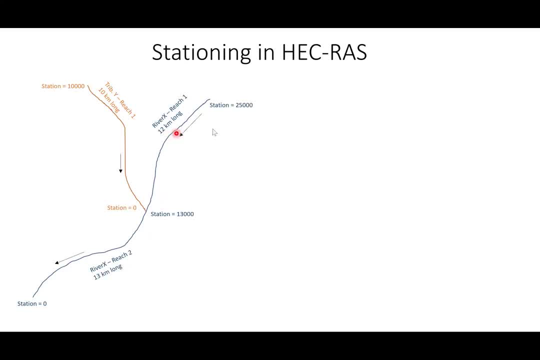 going to be 13 kilometer plus 12 kilometer, which is 25,000 meters now, since this tributary is a different river, so the stationing again will start at zero at the junction and as we go up it will increase. so at the most upstream. 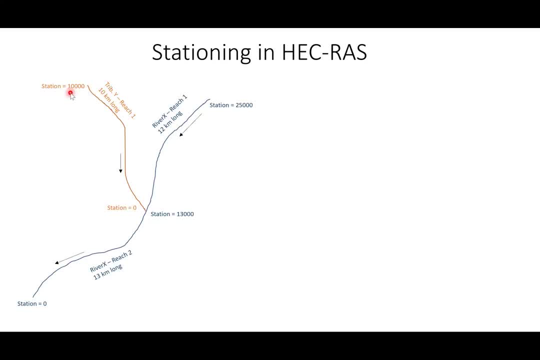 point on this tributary, it will have a stationing of 10,000. so this is how stationing work for the river reaches. now let's assume that we have three cross sections in this river system, so one cross section for each reach, and let's assume that this crossections are. 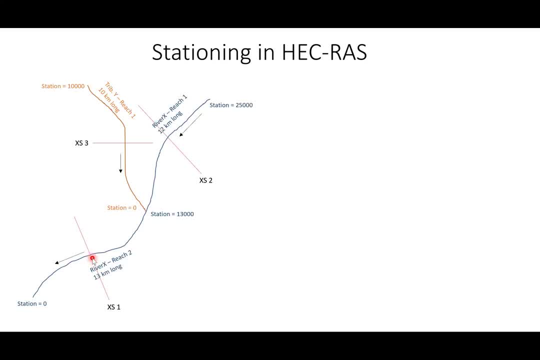 located at the middle of each reach. so the way Harrywood stores information about the location of this cross section is on which river, river which reach within that river and what the stationing is for each cross section. so we have three cross sections and this is how HECRAS will store information. 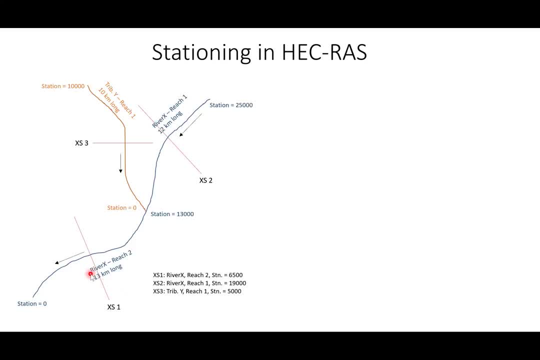 about those. so XS1, which is this cross section, it is located on river X reach 2 and it has a stationing of 6500, since this is the middle of 13,000 long reach. XS2, which is this cross section, it is located on river X reach 1. 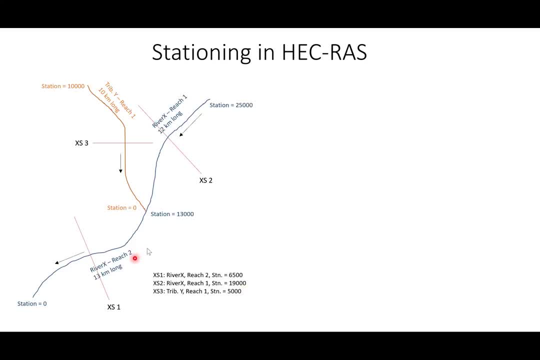 and it has a stationing of 19,000. so 19,000 means 13,000 here, and then half of 12,000, which is 6. so 13,000 plus 6,000 is 19,000. XS3 is on this. 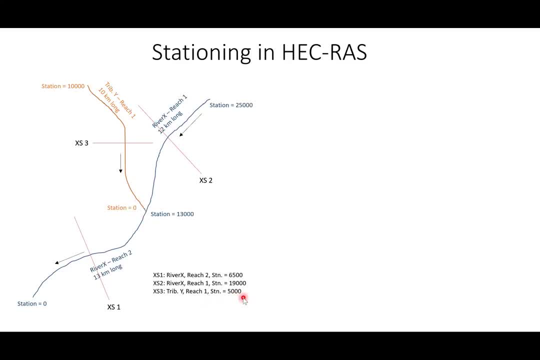 tributary Y reach 1 and it has a stationing of 19,000. so it's again, we are assuming it's- in the middle of this tributary. so this is how HECRAS locates these cross sections, and then each cross section will have: 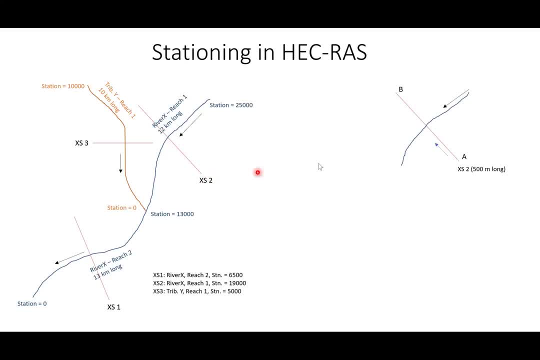 its own stationing. so let's see how that works. so what we see here is XS2, which is this cross section, and when we digitize cross section, we always digitize from left to the right, looking downstream, so the river is flowing in this direction. this 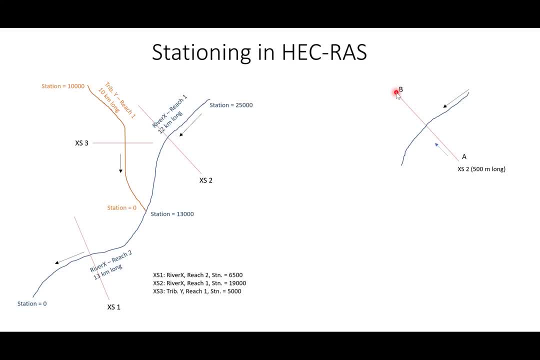 A is our beginning point and B is the end point, and this cross-section will have a ground profile and this is how the stationing for cross-section profile works. so this point A, which is this point, it will have a stationing of zero, because that's where the cross-section start and then there is a elevation. 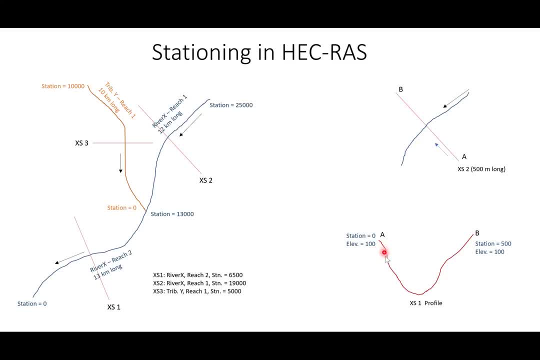 value associated with that. so this cross-section is going to have multiple points along this profile and all of these points will have a station value and elevation value, which I did not list here. and at B, which is our end point, the stationing is 500, because this cross-section is 500 meter long and 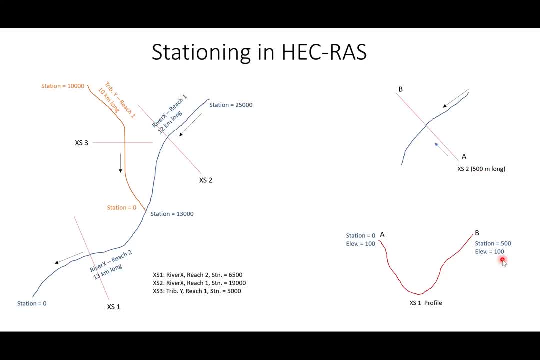 again, it will have elevation associated with it, and in this case we assume that A and B are at the same point and B are at the opposite of it, and so B will have same elevation, which is 100.. So this is how stationing works in HEC-RAS, and now that we 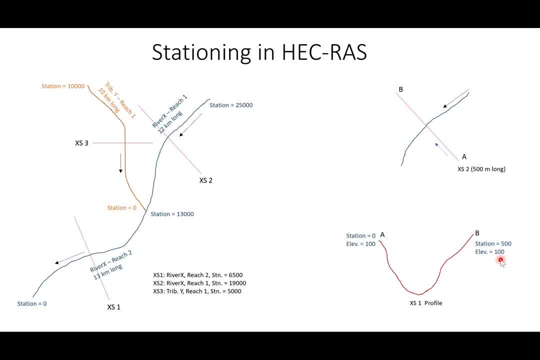 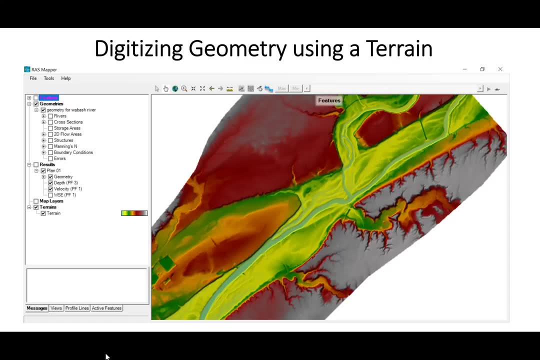 know how it works. let's see how the geometry gets created. As I mentioned earlier, geometry is created in newer version of HEC-RAS using RAS mapper, and which is what you see here on this slide. in order to create geometry, you need a terrain, so this is our digital elevation model for a. 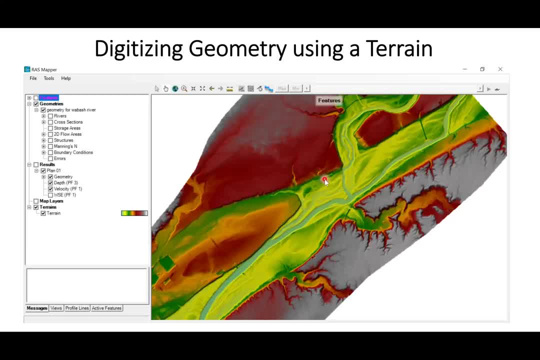 study area. in this case this is Wabash river near Lafayette in Indiana, USA. So you start with a digital elevation model. the first geometry that we digitize is our river center line to establish that reach and river connectivity. so this is our Wabash river upstream, reach downstream. 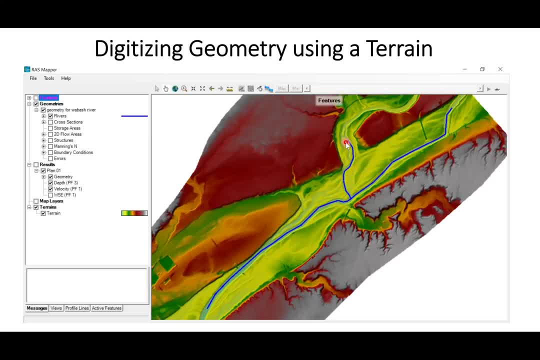 reach. this is a tributaries. this tributary is also a river and it is called Tippecanoe. After we create these reaches, the next geometry that we create is our banks. so these are the bank lines for our river system. after we create bank lines, we create flow paths, and after we create 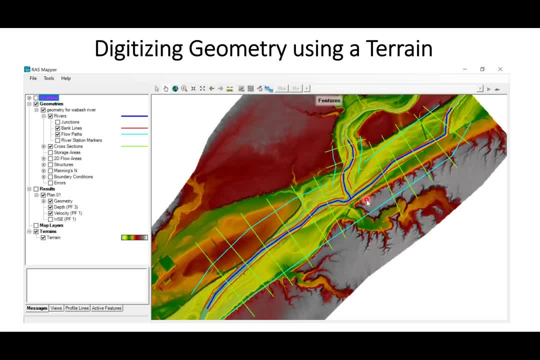 flow paths. we digitize cross sections and if you have any hydraulic structures, you can also incorporate those here. you need to have one cross-section upstream of a hydraulic structure and one cross-section downstream of a hydraulic structure. if you have levees and other hydraulic structures, you can incorporate those two In this module. we will look at how to create a bridge and 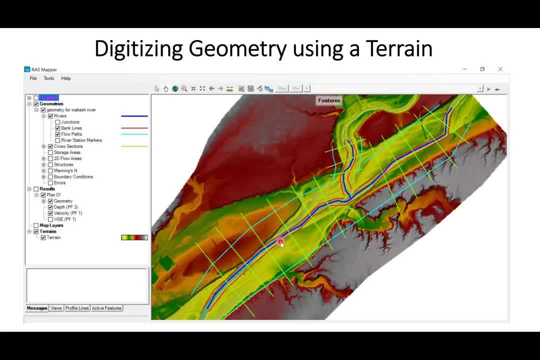 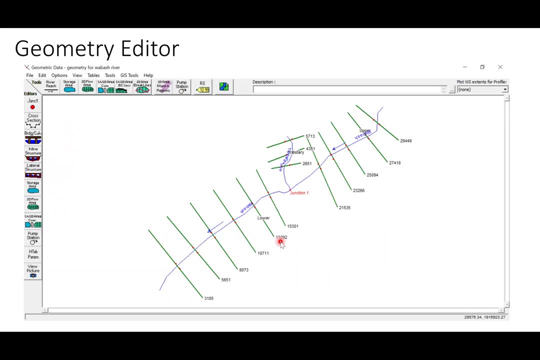 you will learn more about that when we actually do the module. So once you have these basic geometry is defined, then you are ready to create a bridge. So now we will use Wabash river to watch how we create your geometry model. and after you create your geometry model or geometry file, you can edit. 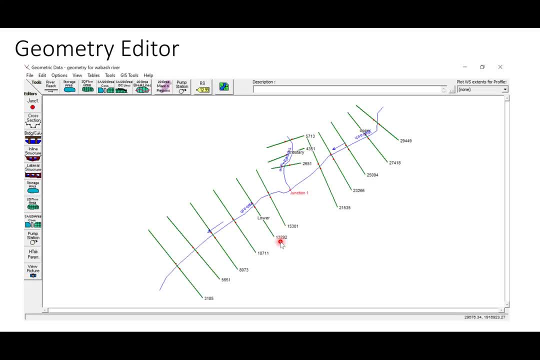 that geometry using geometry editor. so this is how the geometry looks like in geometry editor. so these are our reaches, these are our cross sections. you don't see the bank lines and flow paths. you can see these dots, so they are defining the banks for each cross section. and you can also look at the 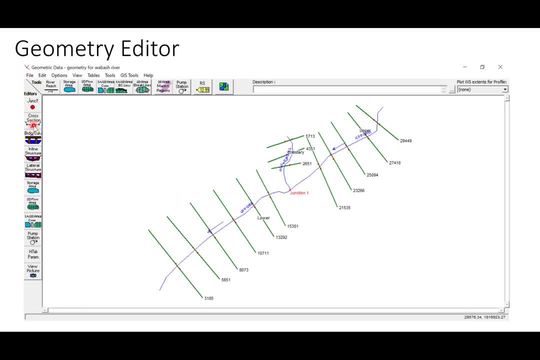 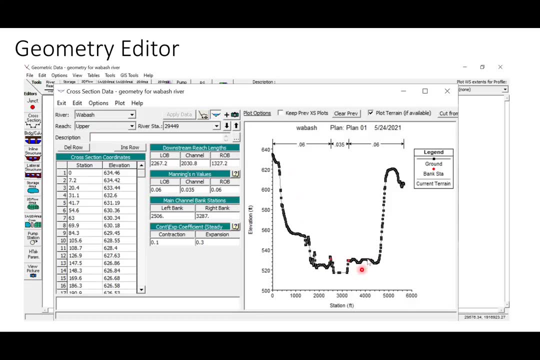 cross section profile by using this cross section editor and if you click on that, this is how it will look. so this is our cross section profile and you can see the station and elevation associated with this profile. so these values are used to show this profile. these are our bank points. 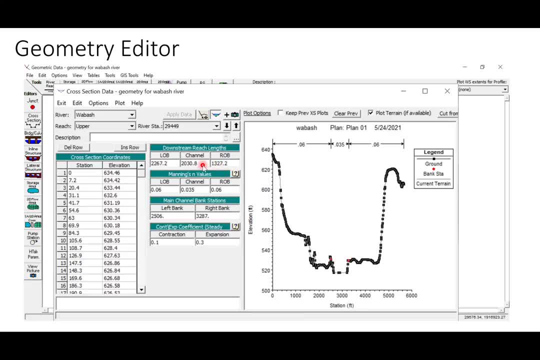 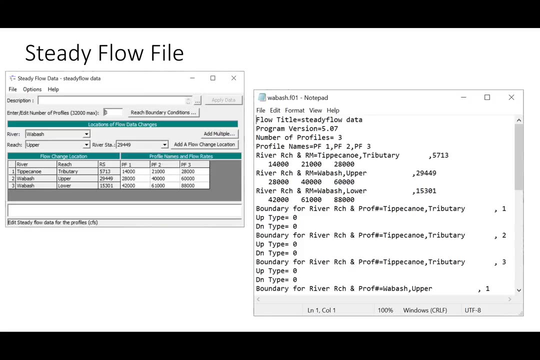 then there is this lob rob channel. all this will be explained when we create the geometry for wabash river in this module. after we create geometry, the next file that we create is a steady flow file. so, since we are performing a steady flow simulation, we will be creating a steady flow file. 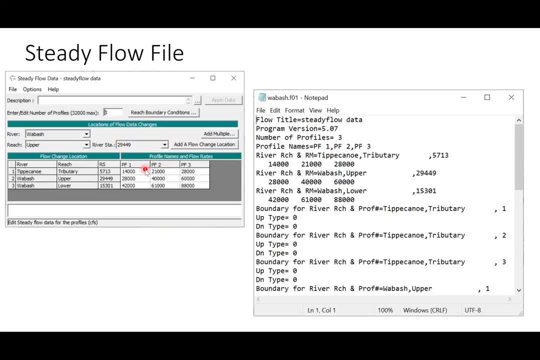 and this is how the interface looks, and what you see here are three profiles. you, So we have three reaches, and for each reach we need an upstream boundary condition and downstream boundary condition. So PF1 stands for profile 1, PF2 stands for profile 2, PF3 stands for profile 3.. 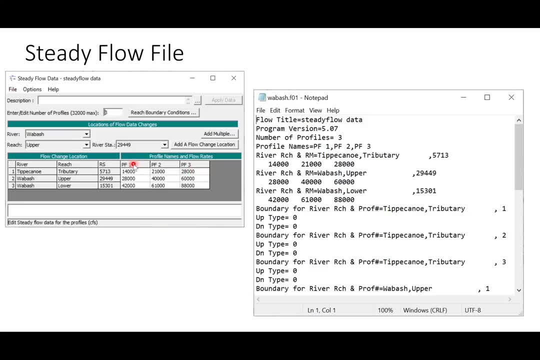 So each profile basically means a simulation for a particular flow. In this case we are performing three simulations, So all you need is one profile. but if you want to perform the simulation for multiple flow values, you create a profile for each flow And this is the text file that gets created after you input this information in this interface and you can see the link between the values that are entered in this interface and how they get stored in this text file. 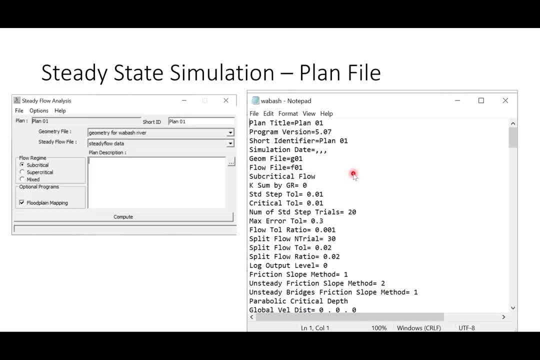 After the steady flow file, we are ready to run the simulation. So plan file gets created when we create a simulation. So in this case we are creating a steady state simulation and we have to specify what kind of flow regime we want to include in the simulation. 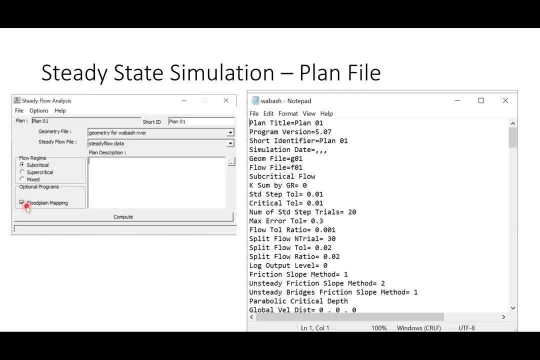 If you want to do the floodplain mapping after simulation, you can check that box and you can see how all this information gets stored in this plan file, which is basically a text file. So the name is plan 01, which is what you see here. 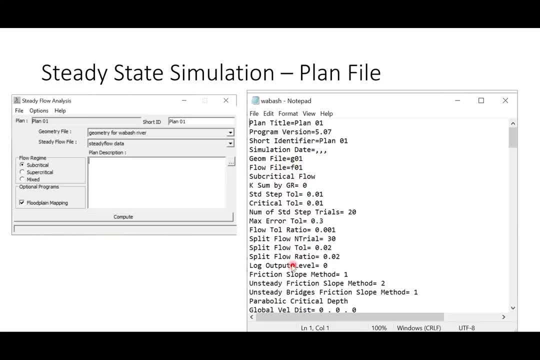 and it will know what geometry file to use. and these are all the default options that the program is going to use in performing the hydraulic simulation. So when we create a simulation you have to run the simulation by using this compute button. Then you may ask what goes on when you hit that compute button. So when you create a simulation, you have to run this simulation by using this compute button, as I mentioned earlier. we are not going to run the simulation right away. When you are going to run the simulation, you are not going to run the simulation for at least a single on a balloons or any other functions. 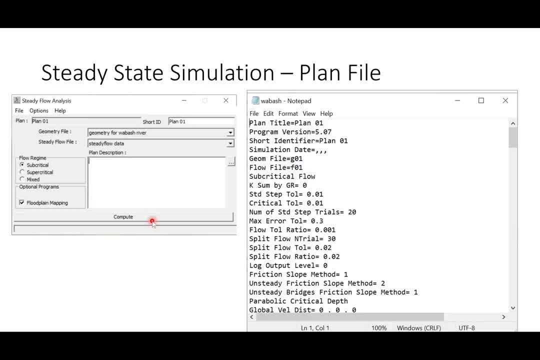 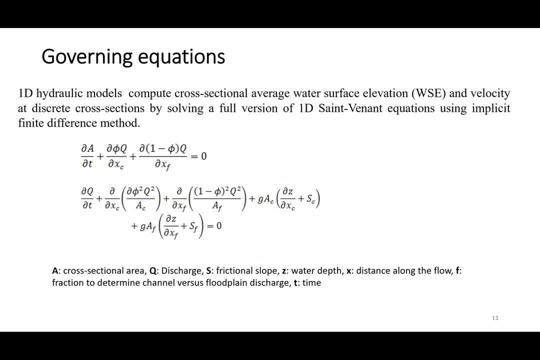 going to go into details of all the hydraulics, but I will give you a quick overview of what is going on, since we are performing a one-dimensional hydraulic simulation. it will use one-dimensional form of Saint-Venant equations, which is what you see here on this slide, and for a steady-state, 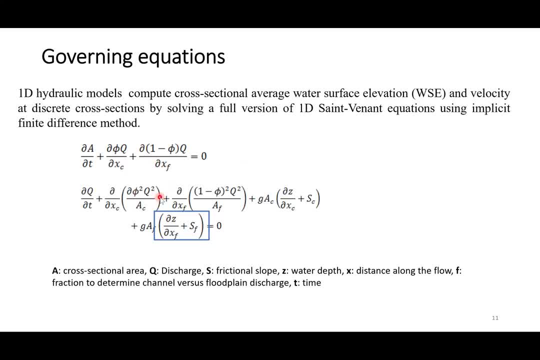 one-dimensional simulation, all these terms, which are acceleration terms, will go away. basically, we end up with this equation, and what this says is the change in water depth with respect to distance, which is X plus the friction slope, is equal to zero. if you know the friction slope, you can find the change. 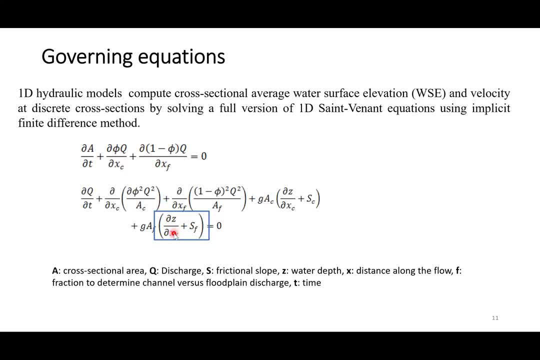 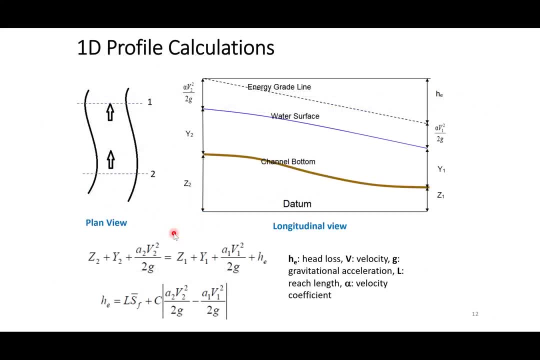 in water surface elevation or flow depth. so the question, then, is: how do we calculate that friction slope? in order to calculate the friction slope, you need to calculate the friction slope. in order to calculate the friction slope, the program uses this energy equation. so, again, assuming that you have some, 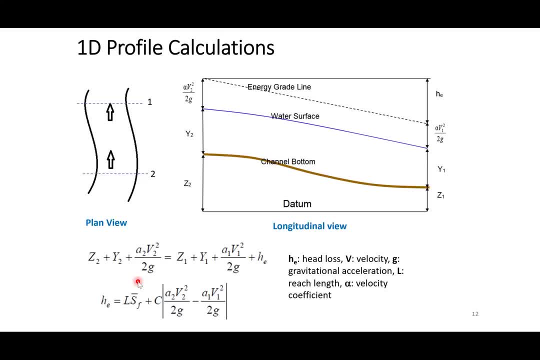 knowledge in hydraulics and open channel flow. so this is the energy equation. so all you have to do is find this head loss and if you know the head loss and the length between two cross-section, you can find out the friction slope. and what you see here is the water surface elevation and the friction slope, and 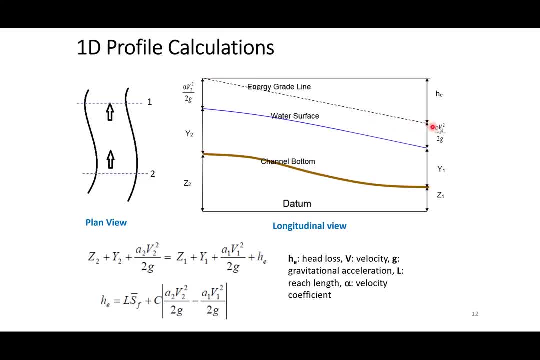 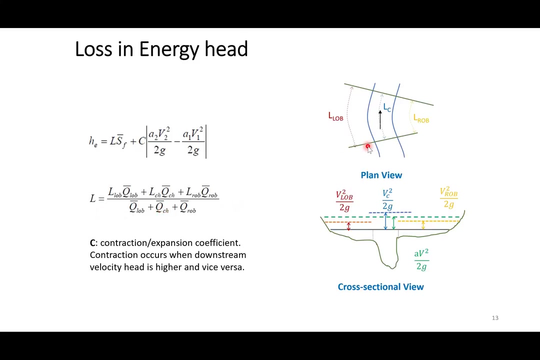 the surface profile and the energy grade line. so all we have to do is find the head loss, and that head loss you can calculate if you know the friction slope and L. then the question is, how do we get this L and SF? this is the expression that HEC-RAS uses to calculate the length between two cross-sections, and 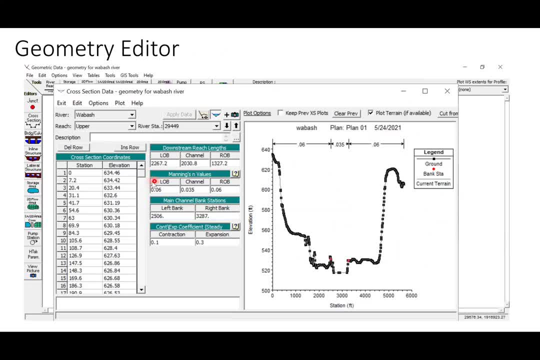 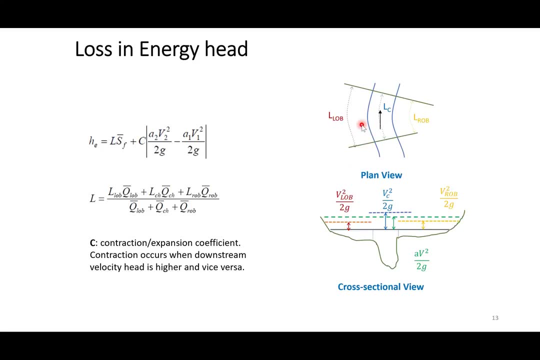 when we look at the river geometry here, we can see that this is the surface. Cao SBOh, mine. yeah, this is the surface and the power plant, which is the pressure at the diameter of the surface. all right, so L, C, h is for the amount of water flowing through this very big surface. that does all. 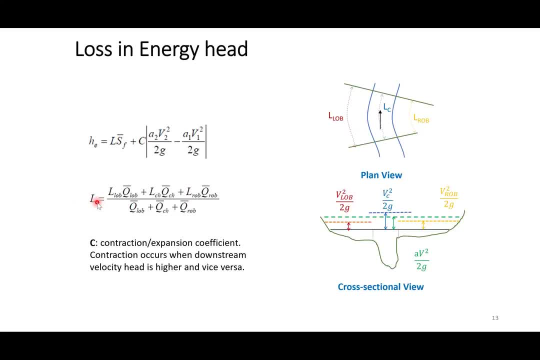 of this work is know. another thing that you need to know is this L, so this L Right here. so you see L O B, which stands for left over bank, this is right over Bank and this is the length along that channel. so L O B, R O B and. 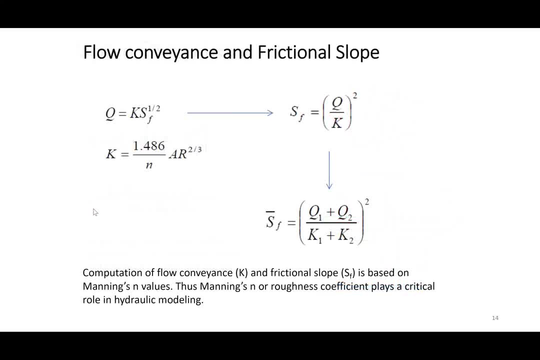 channel, which is what you see here, then you have to calculate the friction slope. and to calculate the friction slope it uses Manning's equation. so this is the flow conveyance and n is the Manning's roughness coefficient. so by using the flow value and the conveyance, 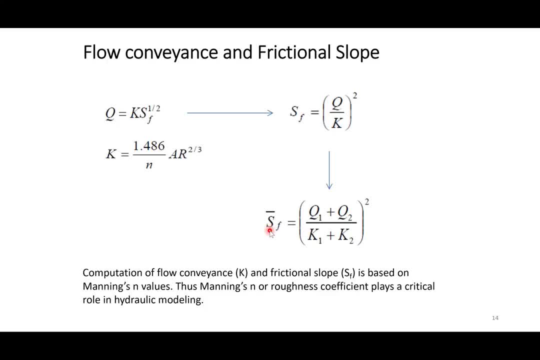 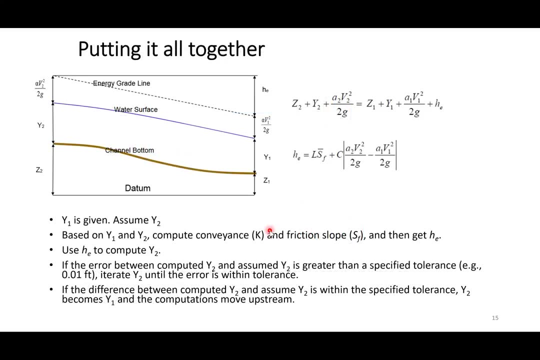 we can find the friction slope between two cross sections. once you know the friction slope, once you know L, then you can find head loss. so now we have all this information, we can put all this together. so the way HEC-RAS works is it solves that one-dimensional Saint Venant equation and energy equation between two. 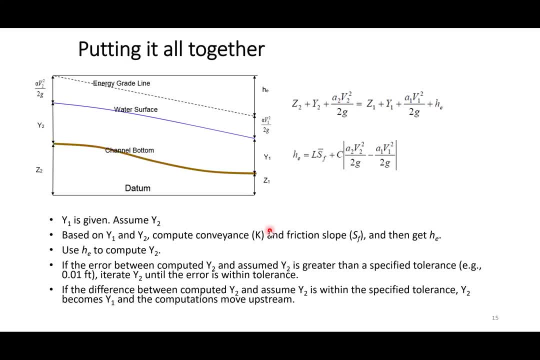 cross-section. since we specify the upstream and downstream boundary condition, we can start at the most downstream cross-section, where we will know what the flow depth is. we will name that cross-section as 1 and we know why 1, what y1 is. so you move up to the next cross-section where you don't know what. 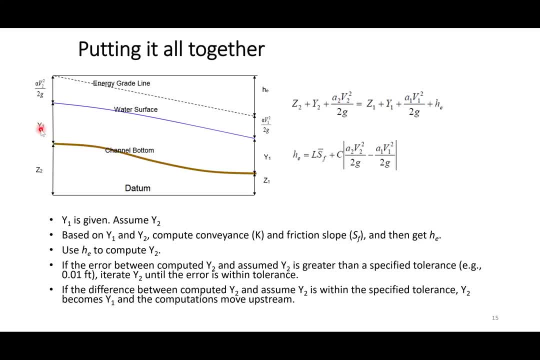 y2 is. so what you do is you assume y2 and then, based on that assumed y2, you find out the flow, conveyance, friction, slope, head loss, and then you solve for y2. if your y2 is same as what you assumed, then you are good, then you don't. 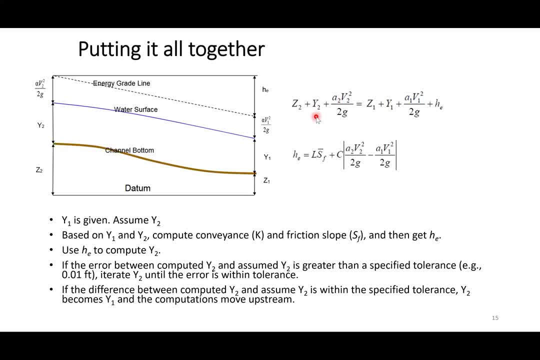 have to do anything. you move on to the next cross-section. if your y2 is not the same as what you assumed, you come back and you keep iterating until you're assumed and calculated y2 are same. once that happens, then your y2 becomes y1 and then the upstream cross-section becomes. 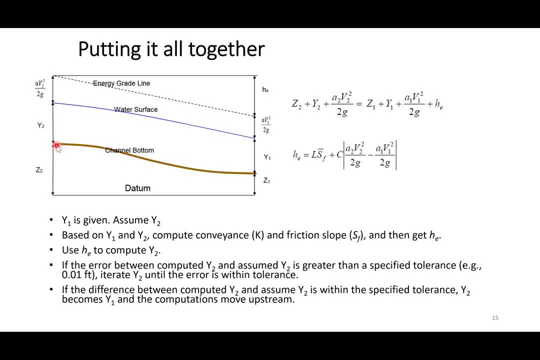 y2, and then you keep doing this until you solve this for all the cross-section. so this is how hydraulic simulations are performed in HEC-RAS, as I mentioned. this is a very quick overview of what is happening, and after the simulation is done, what you end up getting is the water surface elevation. 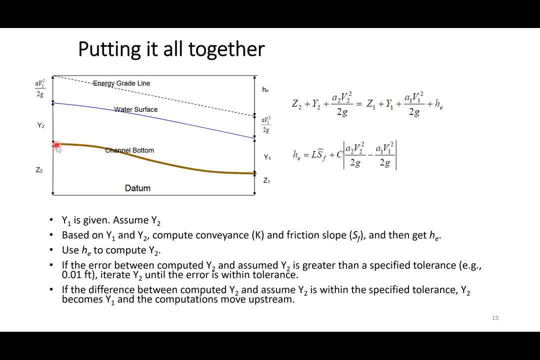 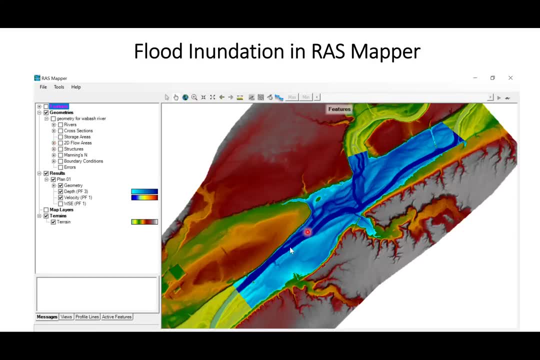 and velocity at each cross-section, which you can interpolate to come up with this flood inundation map. so what you see here is water depth map in RAS mapper, and what we are going to do in this module is create a hydraulic model for Wabash River, perform a 1D simulation and look at the flood inundation map. so I